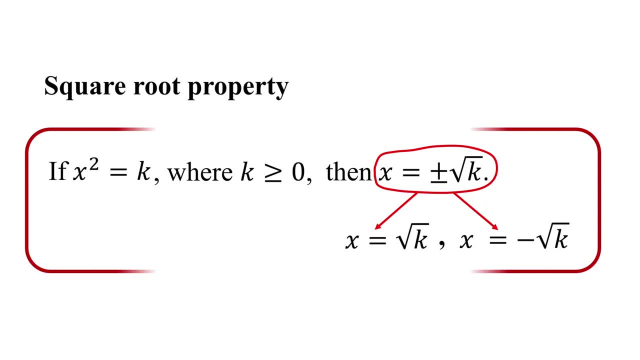 equals the negative of the square root of k. Let's now apply this property to solve these quadratic equations. Our first equation is: x squared equals 49.. By applying the square root property, we find that x equals plus or minus the square root of 49.. 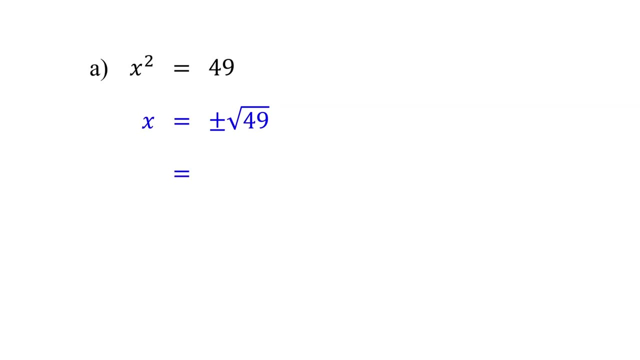 Next, we simplify the square root. The square root of 49 is 7,, right? Therefore, the solutions are x equals 7 or x equals negative 7.. We can check our answers by substituting them back into the original equation. Substituting 7, 7 squared is 7 times 7, which equals 49.. 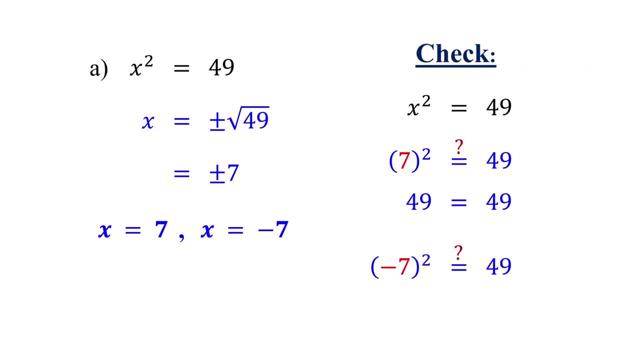 Likewise substituting negative 7, negative 7 squared is negative 7 times negative 7, which also equals 49.. As you can see, both 7 and negative 7 check out, confirming that they are indeed solutions to the quadratic equation. In this example, the coefficient of the quadratic term is 1,. 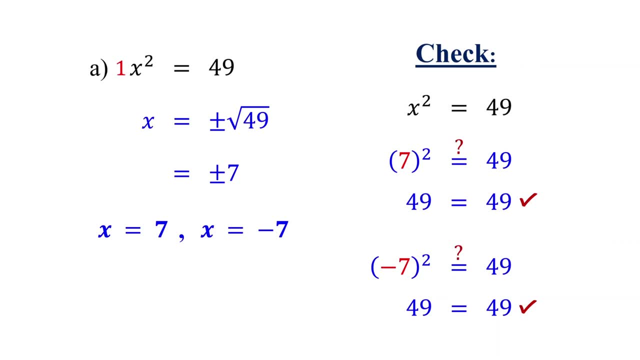 and we were able to apply the square root property directly. But what if the coefficient is not 1?? To apply the square root property, the coefficient of the quadratic term must be equal to 1.. So our initial step in this example is to divide both sides of the equation by 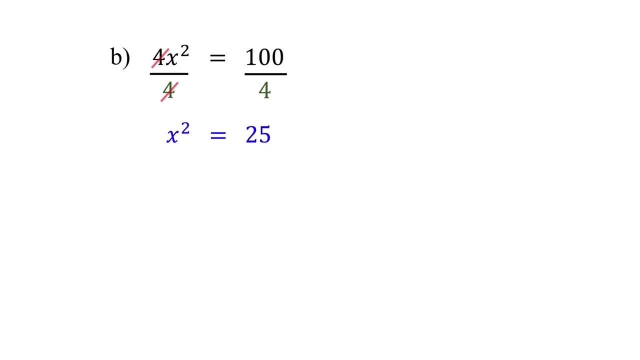 4.. These cancel out and we are left with x squared equals 25.. Now we can apply the square root property, which gives us x equals plus or minus the square root of 25.. Next, simplify the square root. The square root of 25 is 5, so the solutions are: x equals 5 or x equals negative 5.. 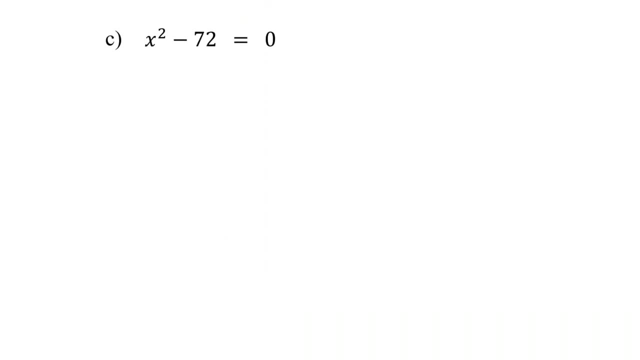 In the next example the quadratic term is not isolated. So what should we do To apply the square root property? the quadratic term must be isolated. So our initial step in this example is to add 72 to both sides of the equation. These cancel out and we get x squared equals 72.. 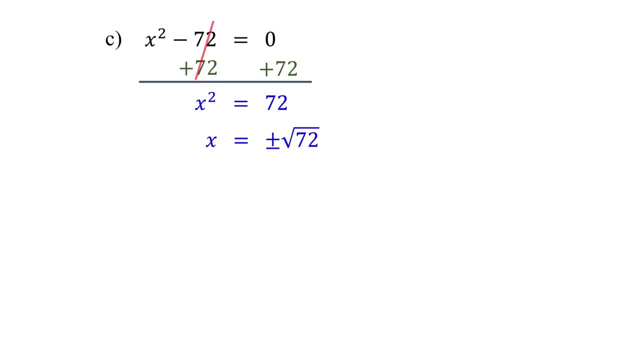 Now you can apply the square root property and you get x equals plus or minus the square root of 72.. The next step is to simplify the square root. 72 is not a perfect square, but it can be written as the product of 36 and 2.. So we can apply the square root property and we get x equals plus or. 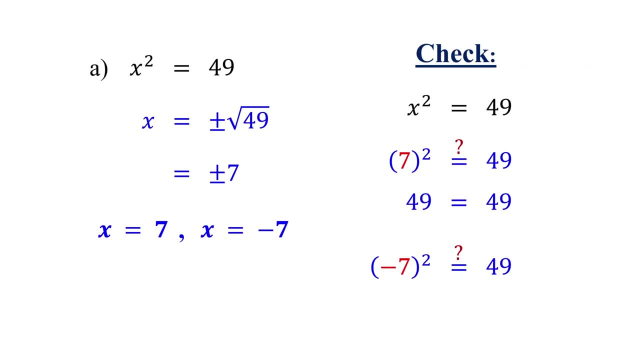 negative 7, negative 7 squared is negative 7 times negative 7, which also equals 49.. As you can see, both 7 and negative 7 check out, confirming that they are indeed solutions to the quadratic equation. In this example, the coefficient of the quadratic term is 1, and we were able to 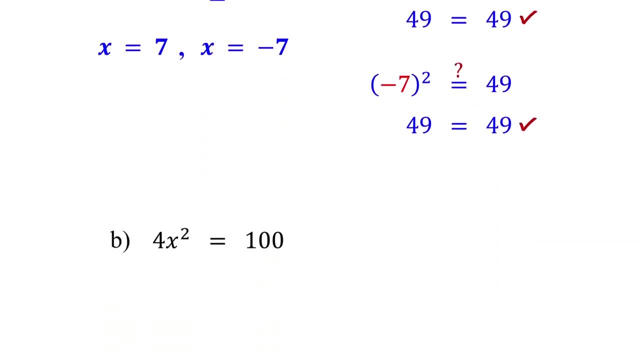 apply the square root property directly. But what if the coefficient is not 1?? To apply the square root property, the coefficient of the quadratic term must be equal to 1.. So our initial step in this example is to divide both sides of the equation by 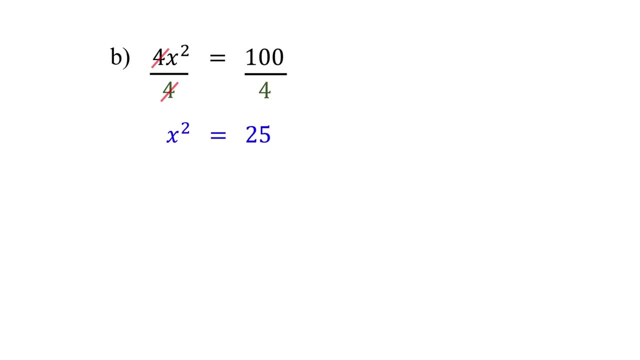 4.. These cancel out and we are left with x squared equals 25.. Now we can apply the square root property, which gives us x equals plus or minus the square root of 25.. Next, simplify the square root. The square root of 25 is 5, so the solutions are: x equals 5 or x equals negative. 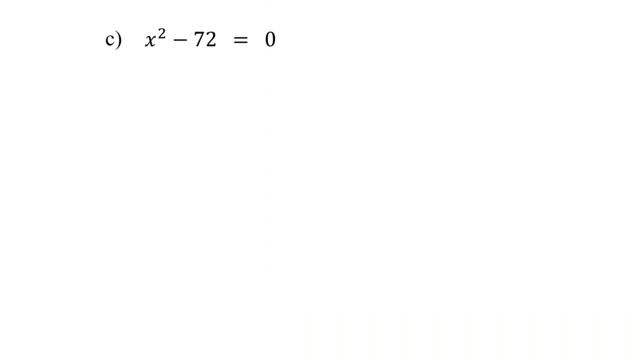 5. In the next example, the quadratic term is not isolated. So what should we do To apply the square root property? the quadratic term must be isolated. So our initial step in this example is to add 72 to both sides of the equation. These cancel out and we get x squared equals 72.. 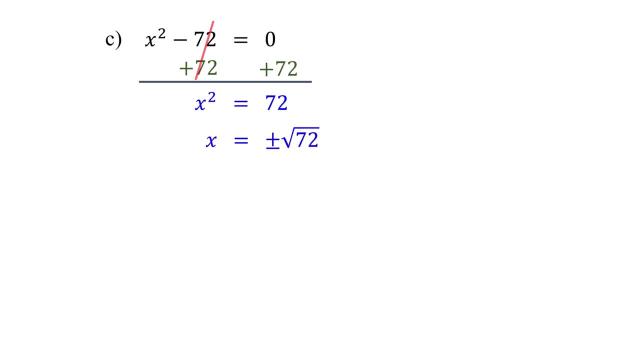 Now you can apply the square root property and you get x equals plus or minus the square root of 72.. The next step is to simplify the square root. 72 is not a perfect square, but it can be written as the product of 36 and 2, right? 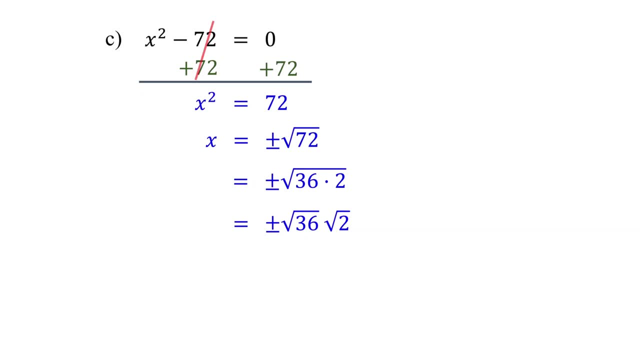 And this is the same thing as the square root of 36 times the square root of 2.. The square root of 36 is 6.. The square root of 2 cannot be further simplified. Therefore, the solutions are: x equals 6 times the square root of 2,. 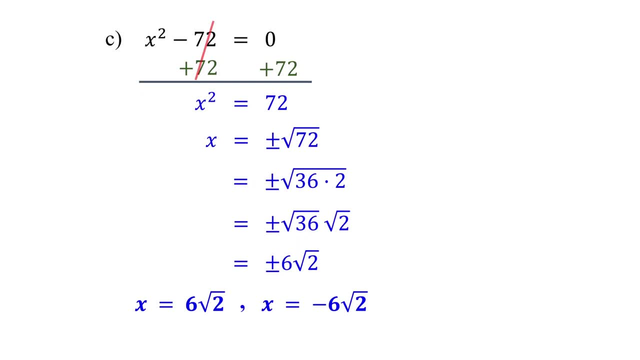 or x equals negative 6 times the square root of 2.. Let's work on another example like this, but a bit more challenging. I encourage you to pause the video and give it a try. Remember to apply the square root property. the quadratic term must be isolated. 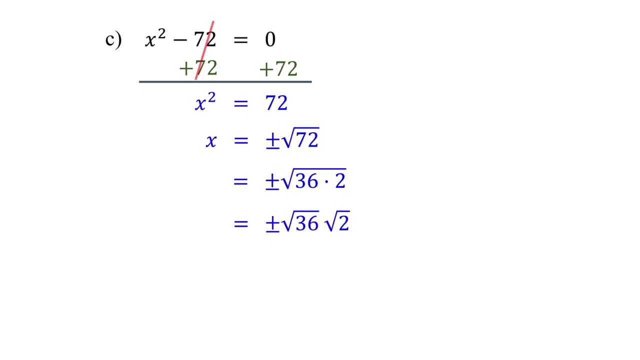 minus the square root of 32, right, And this is the same thing as the square root of 36 times the square root of 2.. The square root of 36 is 6.. The square root of 2 cannot be further simplified. 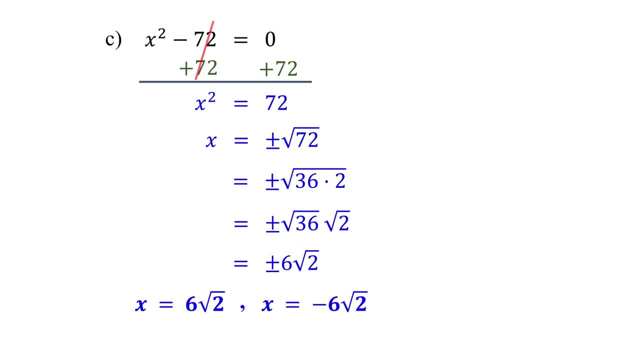 Therefore, the solutions are: x equals 6 times the square root of 2, or x equals negative 6 times the square root of 2.. Let's work on another example like this, but a bit more challenging. I encourage you to pause the video and give it a try. 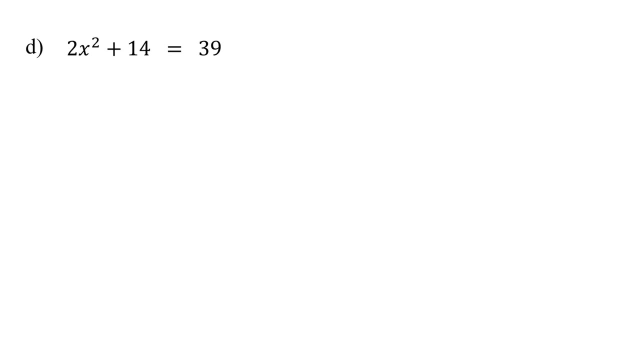 To apply the square root property, the quadratic term must be isolated and its coefficient must be equal to 1.. So first, subtract 14 from both sides of the equation to isolate the quadratic term. Next, divide both sides by 2 to make the coefficient of the. 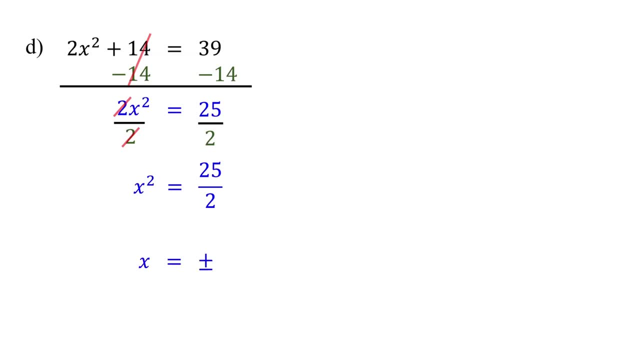 quadratic term 1.. At this point you can apply the square root property. The next step is to simplify the square root. This is the same thing as the square root of 25 over the square root of 2, right, The square root of 25 is 5.. In algebra, when the denominator of a fraction has a radical, 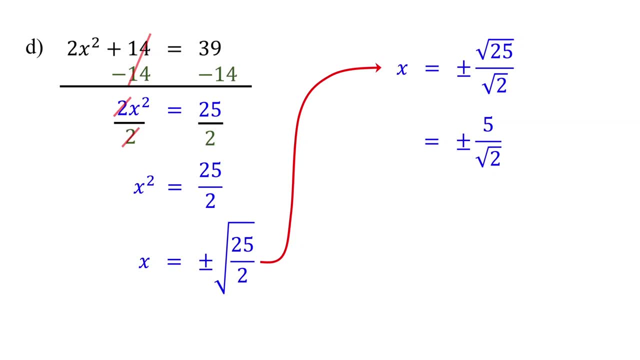 as in this case, it is not considered simplified. So we need to rationalize the denominator. to simplify it, Multiply both the numerator and the denominator by the square root of 2.. In the numerator, you have 5 times the square root of 2.. In the denominator, 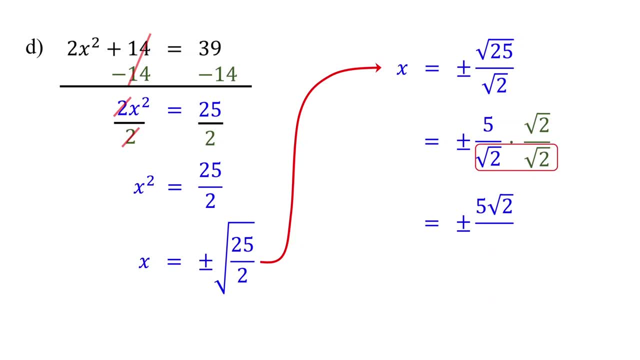 the square root of 2 times the square root of 2 is the square root of 4, which equals 2.. Therefore, the solutions are: x equals 5 times the square root of 2 over 2, or negative, 5 times the square root of 2 over 2.. At the beginning of the video. 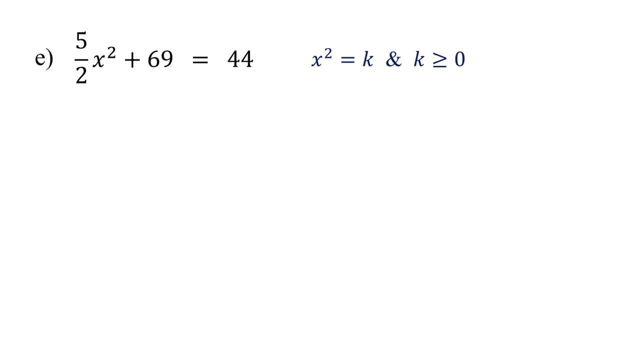 when we defined the square root property, we said that if x squared equals k and k is greater than or equal to 0, then x equals plus or minus the square root of k. But what will happen if k is less than 0? This will be the case in this example. 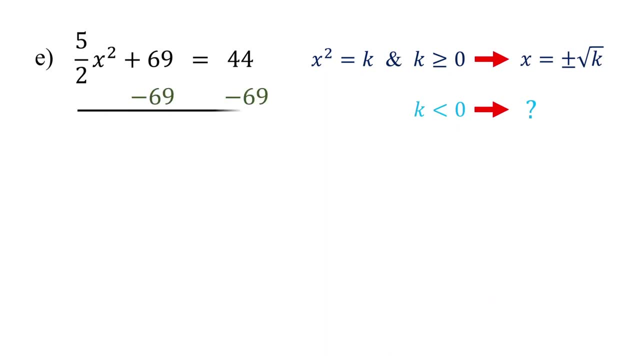 First isolate the quadratic term by subtracting 69 from both sides of the equation. These cancel out, and 44 minus 69 equals negative 25.. Then make the coefficient 1 by multiplying both sides by 2 over 5.. On the left side, the 2s and the 5s cancel each other out, leaving us with x squared. 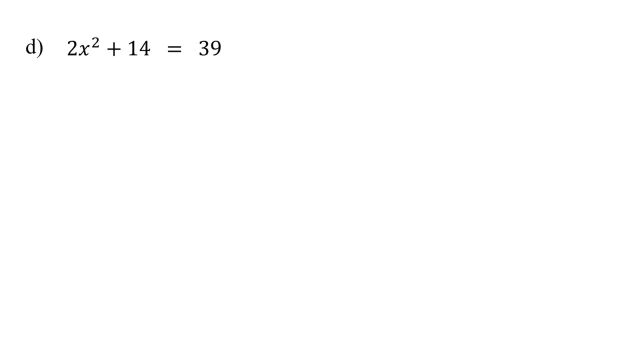 and its coefficient must be equal to 1.. So first, subtract 14 from both sides of the equation to isolate the quadratic term. Next, divide both sides by 2 to make the coefficient of the quadratic term 1.. At this point you can apply the square root property. 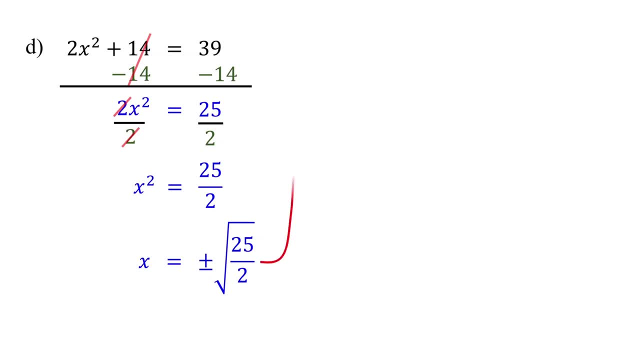 The next step is to simplify the square root. This is the same thing as the square root of 25.. The square root of 25 is 5 over the square root of 2, right. The square root of 25 is 5.. 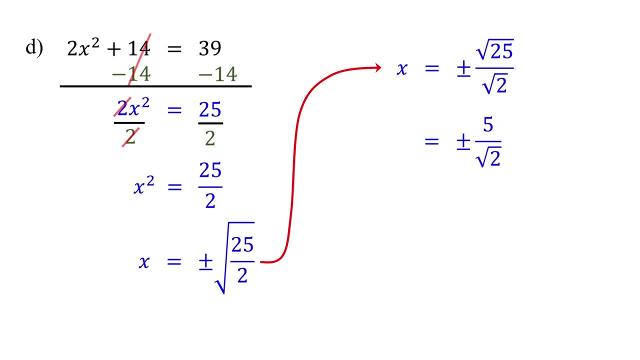 In algebra, when the denominator of a fraction has a radical, as in this case, it is not considered simplified. So we need to rationalize the denominator. to simplify it, Multiply both the numerator and the denominator by the square root of 2.. 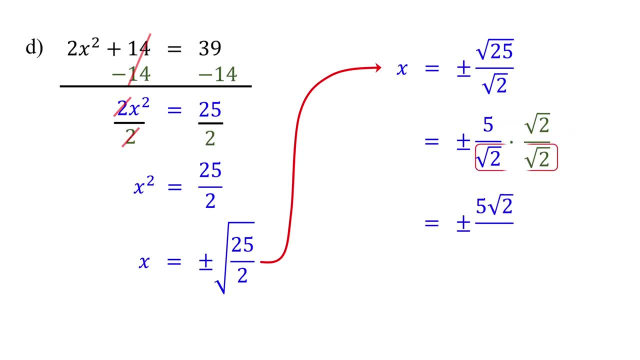 In the numerator you have 5 times the square root of 2.. In the denominator, the square root of 2 times the square root of 2 equals the square root of 4, which equals 2.. Therefore, the solutions are: x equals 5 times the square root of 2 over 2,. 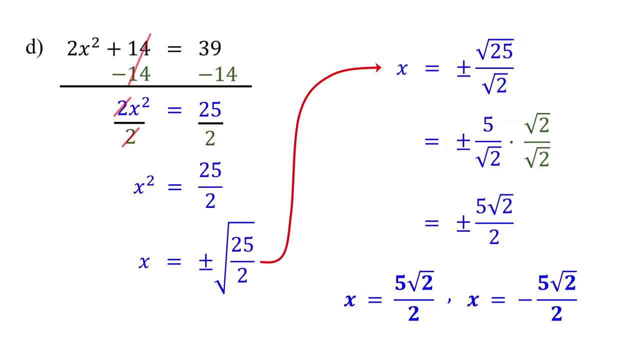 or negative, 5 times the square root of 2 over 2.. At the beginning of the video, when we defined the square root property, we said that if x squared equals k and k is greater than or equal to 0, then x equals, plus or minus, the square root of k. 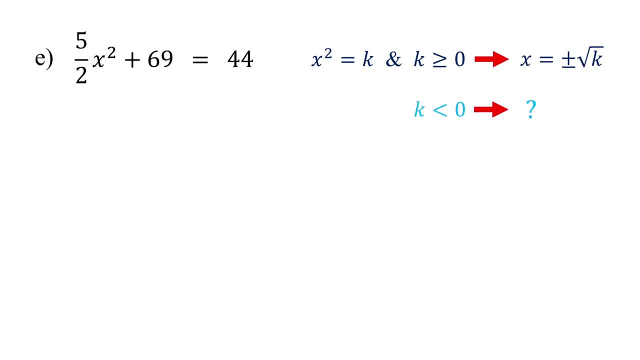 But what will happen if k is less than 0? This will be the case in this example. First, isolate the quadratic term by subtracting 69 from both sides of the equation. These cancel out, and 44 minus 69 equals negative 25.. 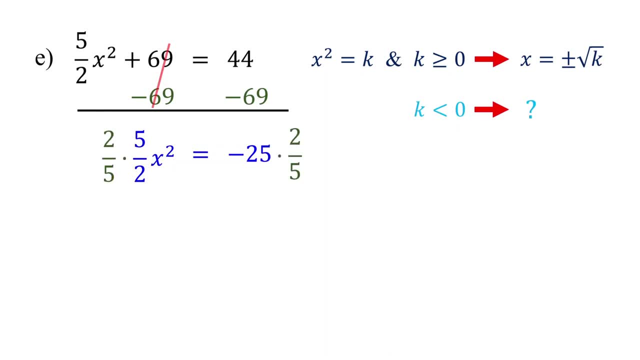 Then make the coefficient 1 by multiplying both sides by 2 over 5.. On the left side, the 2s and the 5s cancel each other out, leaving us with x squared. On the right side, simplify negative 25 and 5 to negative 5.. 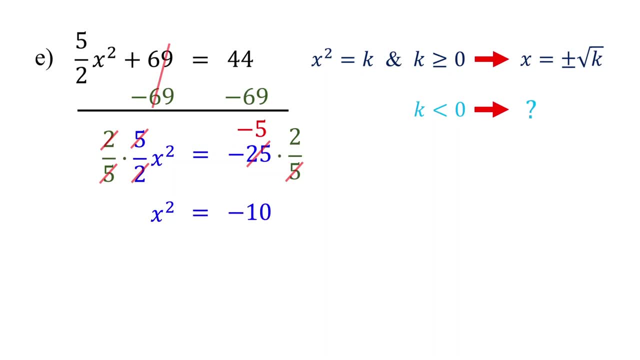 Then multiply negative 5 by 2 to get negative 10.. As you can see now, k is negative. If we apply the square root property, the number inside the square root becomes negative. However, in the real number system we cannot take the square root of a negative number right. 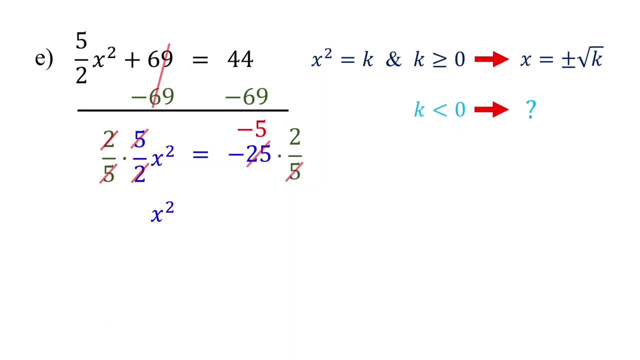 On the right side. simplify negative 25 and 5 to negative 5.. Then multiply negative 5 by 2 to get negative 10.. As you can see now, k is negative. If we apply the square root property, the number inside the square root becomes negative. However, in the real number system, 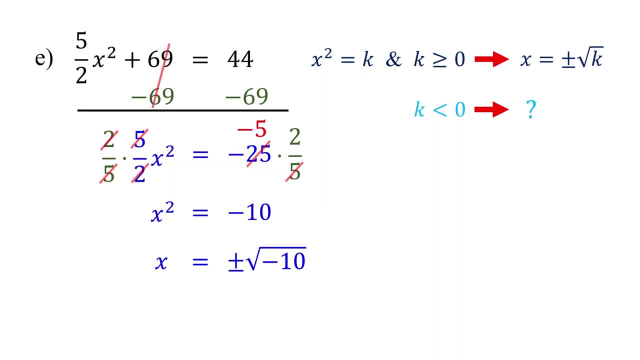 we cannot take the square root of a negative number right. Therefore, the answer to this problem is that there is no real solution In general. if k is less than 0, then the quadratic equation has no real solution. Now let's work on some examples that are a bit more challenging. 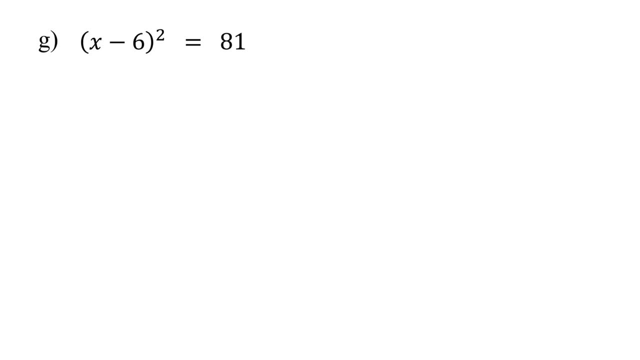 Please stay with me. In this example the squared term is not just x. Instead it is x minus 6.. In such cases, treat the entire binomial as a single variable and apply the square root property directly. So we have x minus 6 equals plus or minus the square root of 81.. The square root of. 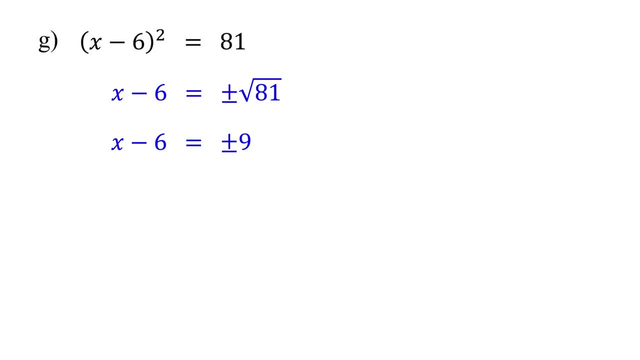 81 is 9, right Now we have two equations: x minus 6 equals 9 and x minus 6 equals negative 9.. The next step is to solve each equation. Let's start with the first equation. Add 6 to both. 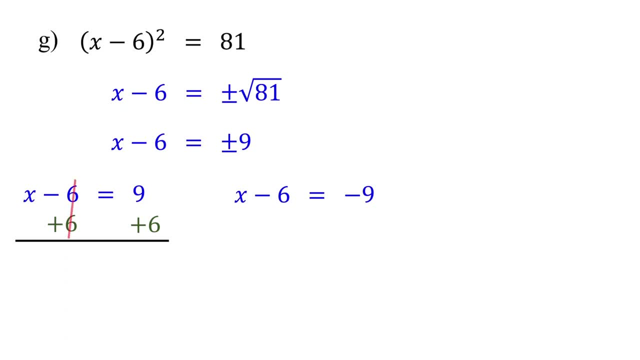 sides to isolate x. These cancel out and 9 plus 6 is 15.. For the second equation, again, add 6 to both sides. Cancel out these Negative. 9 plus 6 is negative 3.. Therefore the solutions: 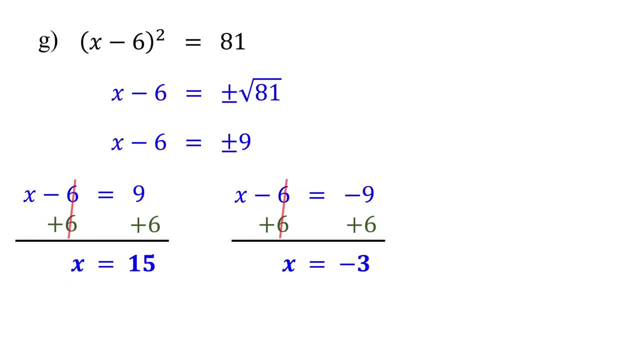 are x equals 15 or negative 3.. Let's verify our solutions by substituting them back into the original equation. Substituting 15,, 15 minus 6 is 9, and 9 squared equals 81.. Similarly, substituting negative 3,: negative 3 minus 6 is negative 9, and negative 9 squared is also equals. 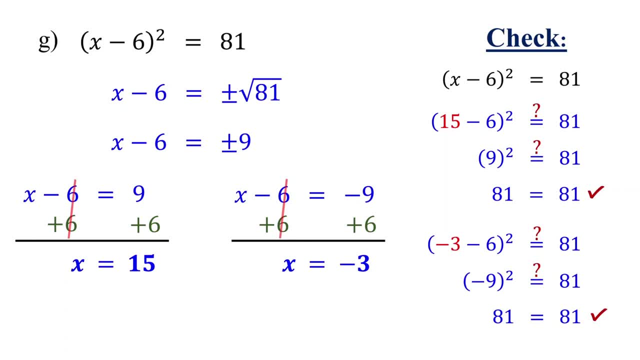 81.. As you can see, both 15 and negative 3 check out, confirming that they are indeed solutions to the quadratic equation. Let's work on another example like this. Just like in the previous example, consider the following: Remember to reduce our solution. 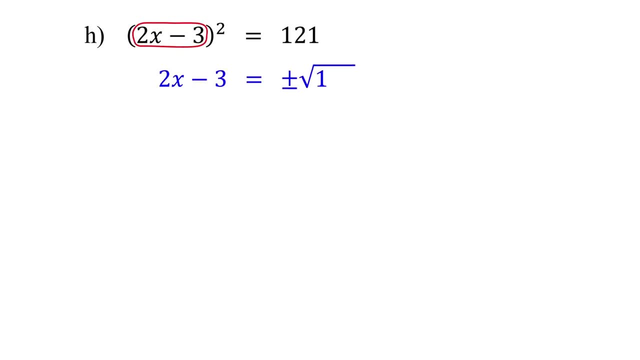 That mean you'll find that both honeymoon masculinity and unemployment is 11, so we will not be able to solve our solution if we don't reduce the solution. In this case, you can read the partition And you can create a solution to solve your solution of. 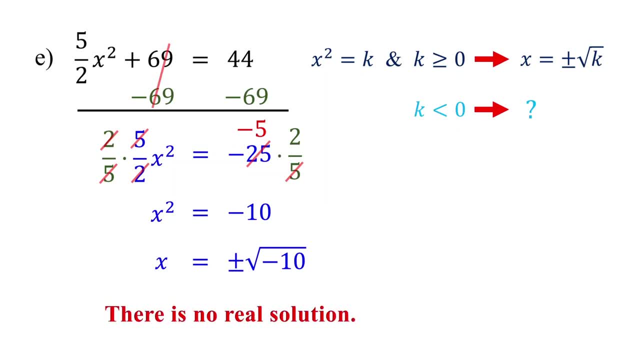 Therefore, the answer to this problem is that there is no real solution In general. if k is less than 0, then the quadratic equation has no real solution. Now let's work on some examples that are a bit more challenging. Please stay with me. 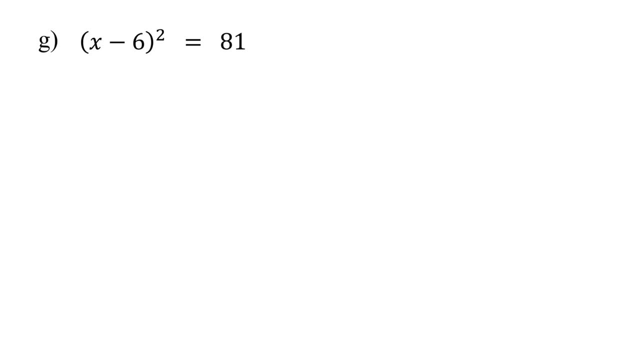 In this example the squared term is not just x. Instead it is x minus 6.. In such cases, treat the entire binomial as a single variable and apply the square root property directly. So we have x minus 6 equals plus or minus the square root of 81.. 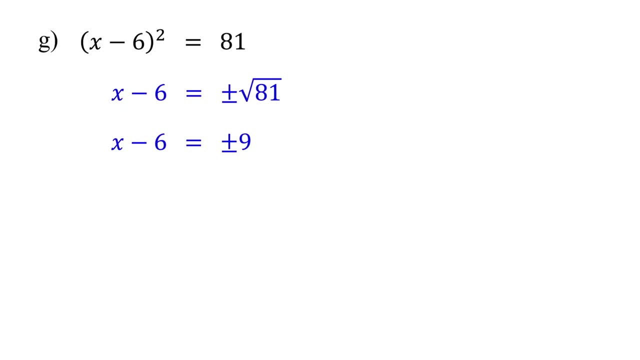 The square root of 81 is 9,. right Now we have two equations: x minus 6 equals 9, and x minus 6 equals negative 9.. The next step is to solve each equation. Let's start with the first equation. 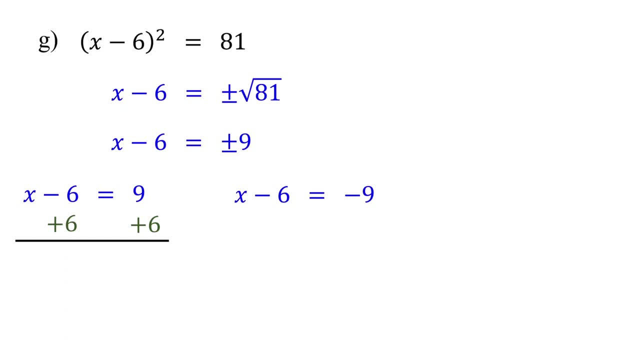 Add 6 to both sides to isolate x. These cancel out and 9 plus 6 is 15.. For the second equation, again add 6 to both sides. Cancel out these Negative 9 plus 6 is negative 3.. 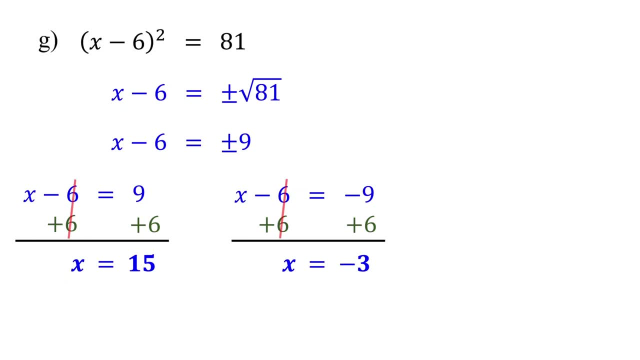 Therefore, the solutions are: x equals 15 or negative 3.. Let's verify our solutions by substituting them back into the original equation: Substituting 15,, 15 minus 6 is 9, and 9 squared equals 81.. 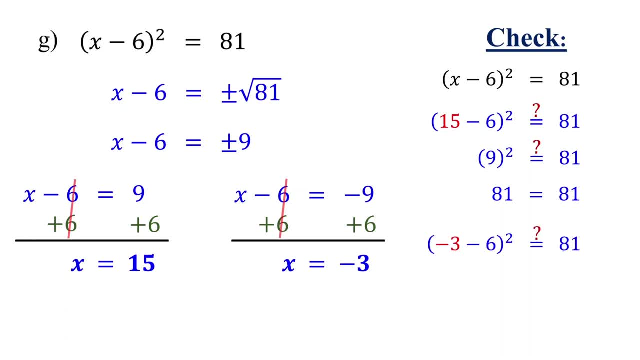 Similarly, substituting negative 3, negative 3 minus 6 is negative 9, and negative 9 squared is also equals 81.. As you can see, both 15 and negative 3 check out, confirming that they are indeed solutions to the quadratic equation. 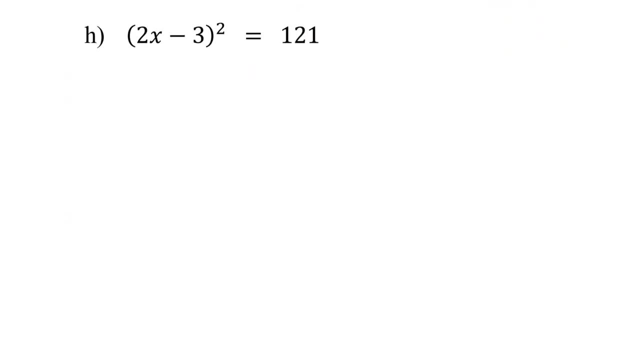 Let's work on another example like this. Just like in the previous example, you can treat the entire binomial as a single variable and apply the square root property directly. The square root of 121 is 11.. Next, write down the two equations and solve them. 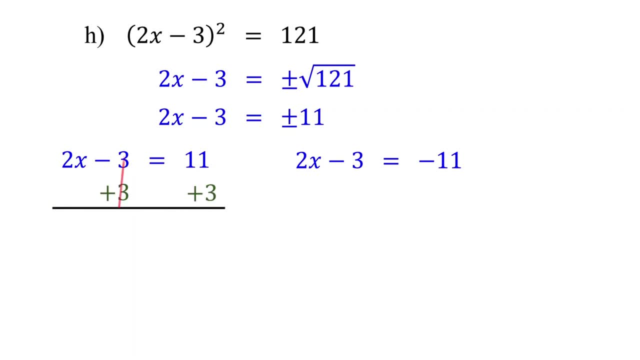 Starting with the first equation, add 3 to both sides of the equation to isolate 2x. Then divide both sides by 2, and you get x equals 7.. For the second equation, again add 3 to both sides of the equation to isolate 2x. sky Bottom and save. Statista will test this Mitsubushi situation. The square root of 21 is 11.. Now we will solve this solution. Make the To ASM gradient via how we would like the solution of the first equation to be. 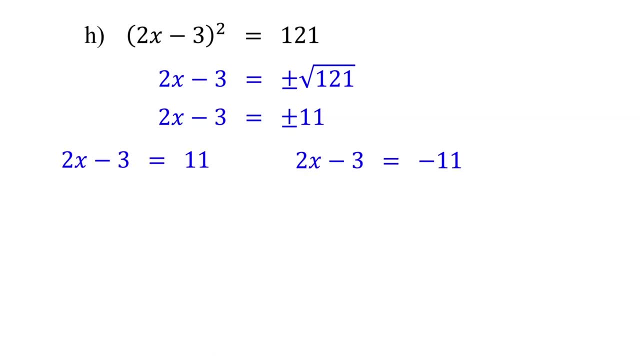 solved. Write down the two equations and solve them. For the first equation, add 3 to both sides of the equation to isolate 2x. Then divide both sides by 2, and you get x equals 7.. For the second equation, again add 3 to both sides of the equation to isolate 2x. 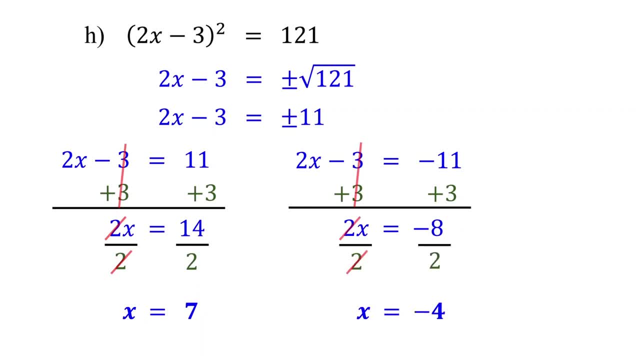 then divide both sides by 2 and you get x equals negative 4.. Therefore, the solutions are: x equals 7 or negative 4.. If you have found this video helpful so far, please give it a thumbs up and consider subscribing. Now it is your turn. 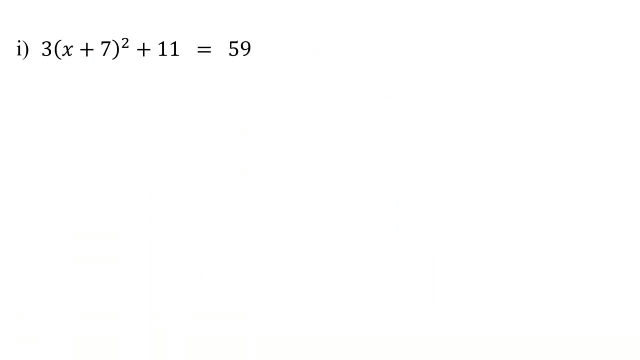 please pause the video and give it a try. Remember to apply the square root property. the quadratic term must be isolated and its coefficient must be equal to 1.. So first, subtract 11 from both sides of the equation to isolate the quadratic term. Next, divide both sides of the equation by 3 to make the 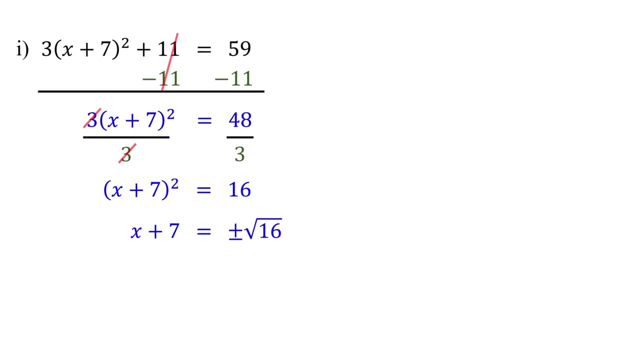 coefficient 1. At this point you can apply the square root property. The square root of 16 is 4.. Next set up the two equations and solve them. From the first equation, you get x equal to negative. 3. From the second equation, you: 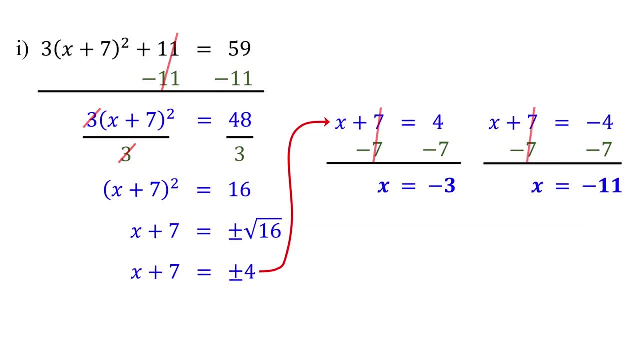 get x equal to negative 3.. Therefore, the two solutions are: x equals negative 3 or negative 11.. Moving on to the next example, the left side of the equation looks a bit different from what we have seen before, but don't worry, it is a perfect square trinomial By: 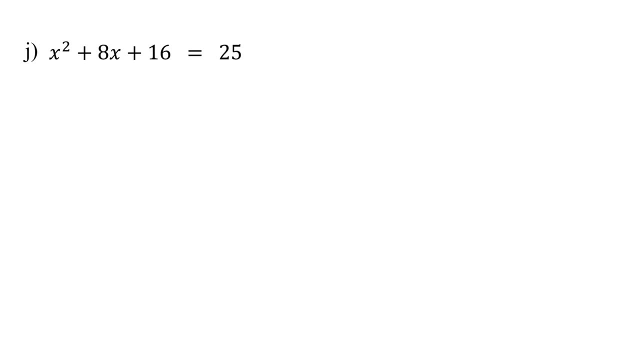 factoring it. we can rewrite it in a familiar form we have been working with, which will allow us to apply the square root property directly. This perfect square trinomial is in the form: a squared plus 2, a, b plus b squared. To recognise if a trinomial is a perfect square, you can follow these three simple. 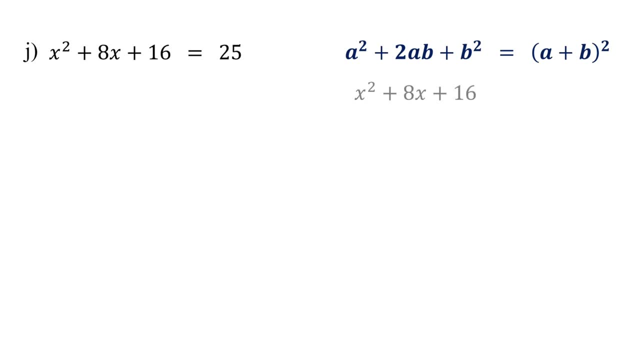 steps. First, check if the first term is a perfect square: x squared is indeed a perfect square. Next, check if the last term is a perfect square: 16 is a perfect square and can be written as 4 squared right. Finally, check if the middle term 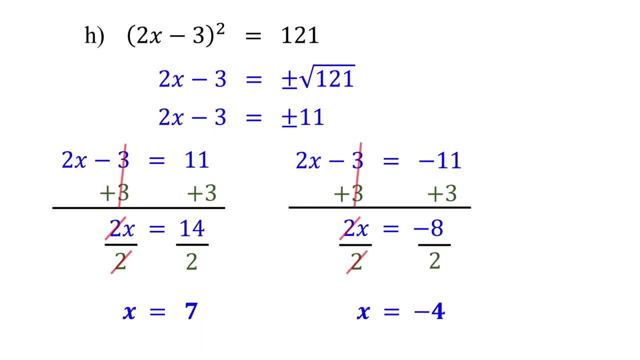 Then divide both sides by 2, and you get x equals negative 4.. Therefore, the solutions are: x equals 7 or negative 4.. If you have found this video helpful so far, please give it a thumbs up and consider subscribing. 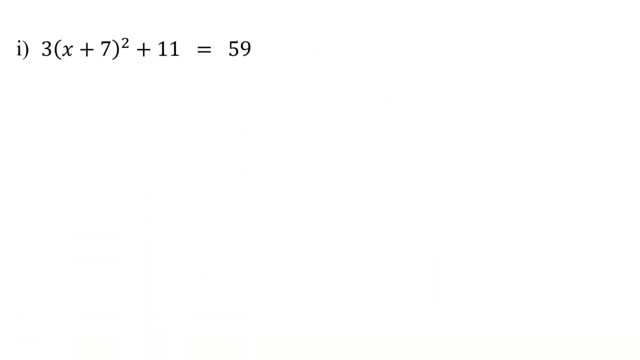 Now it is your turn. Please pause the video and give it a try. Remember to apply the square root property. the quadratic term must be isolated and its coefficient must be equal to 1.. So first subtract 11 from both sides of the equation to isolate the quadratic term. 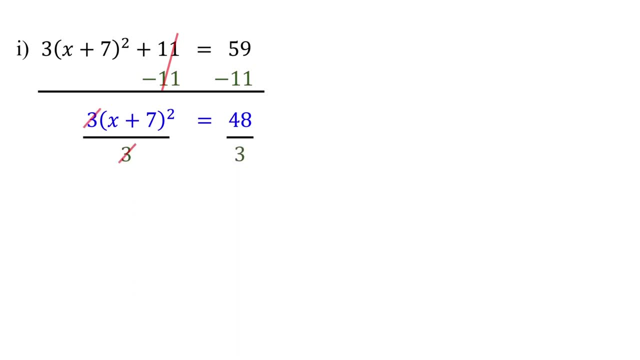 Next divide both sides of the equation by 3 to make the coefficient 1.. At this point you can apply the square root property. The square root of 16 is 4.. Next set up the two equations and solve them. 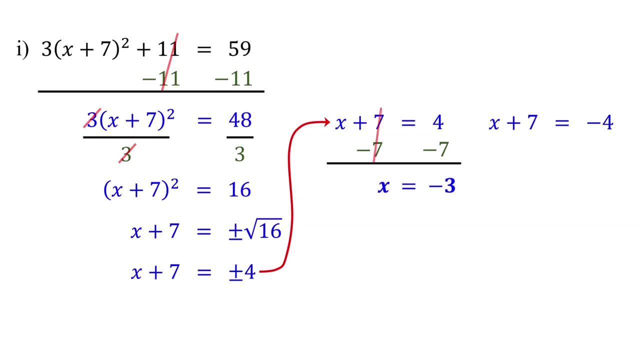 From the first equation, you get x equal to negative 3.. From the second equation, you get x equal to negative 11. Therefore, the two solutions are: x equals negative 3 or negative 11.. Moving on to the next example, 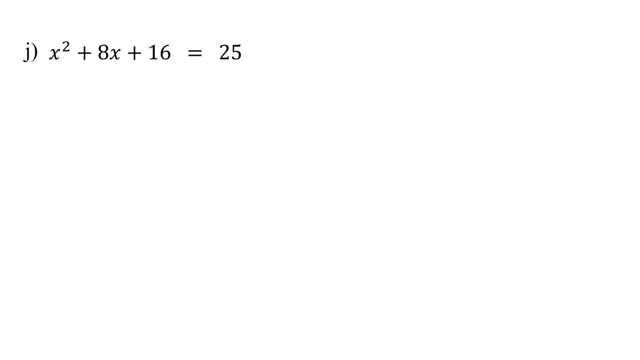 the left side of the equation looks a bit different from what we have seen before, But don't worry, it is a perfect square trinomial. By factoring it, we can rewrite it in a familiar form we have been working with, which will allow us to apply the square root property directly. 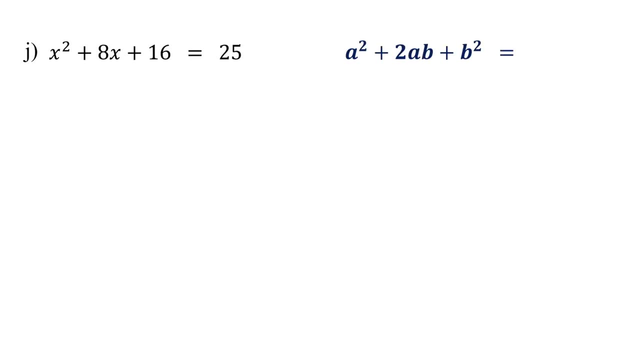 This perfect square trinomial is in the form a squared plus 2ab plus b squared, which is equal to a plus b squared. To recognize if a trinomial is a perfect square, you can follow these three simple steps. First, check if the first term is a perfect square. 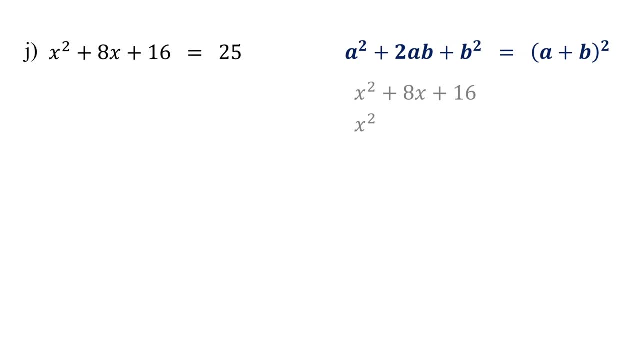 x squared is indeed a perfect square. Next, check if the last term is a perfect square, 16 is a perfect square and can be written as 4 squared right. Finally, check if the middle term is 2 multiplied by a times b. 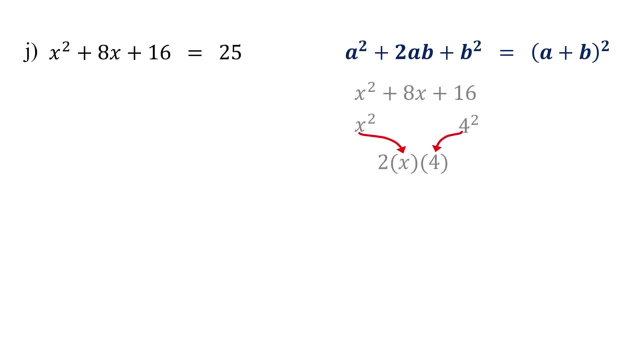 is 2 multiplied by a times b, 2 times x times 4.. The answer is the following: 1 times b times x times 4 is 8x. Therefore, since all three conditions are met, this trinomial is a perfect. 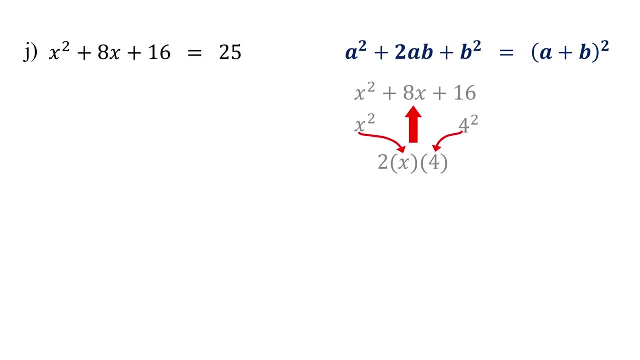 square. Now, since a is x and b is 4, we can factor it as x plus 4 squared. Notice that if the sign of the middle term is positive, the sign in the factor is also positive. Similarly, if it is negative, the sign in the factor is also negative. Now treat the whole binomial. 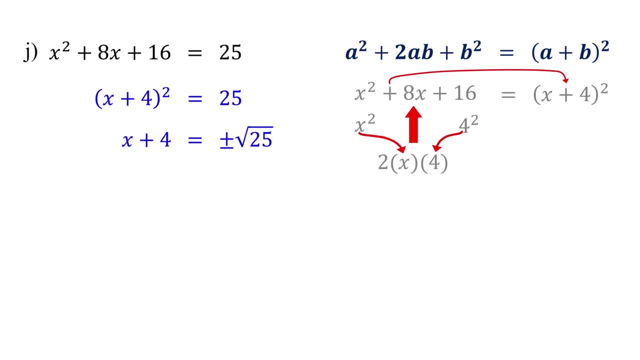 as a single variable and apply the square root property. The square root of 25 is 5.. Next set up the two equations and solve them. From the first equation, we get x equal to 1.. From the second equation, we get x equal to negative 9.. Therefore, the two solutions are: 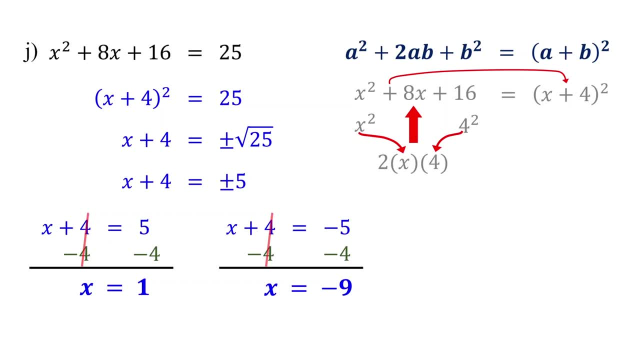 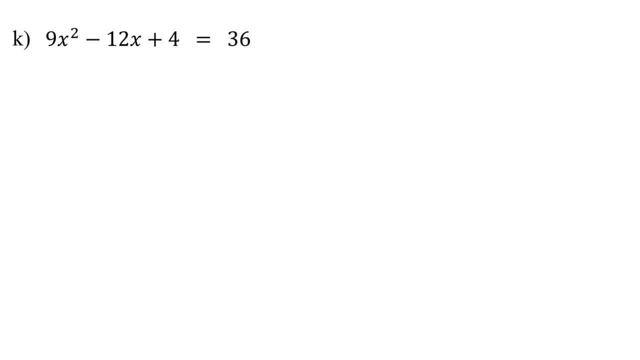 x equal to 1 or negative 9.. Let's do one more example like this. This is the final one, so please stay with me. Just as we did in the previous example, our first step is to factor the perfect square trinomial. This trinomial is in the form: 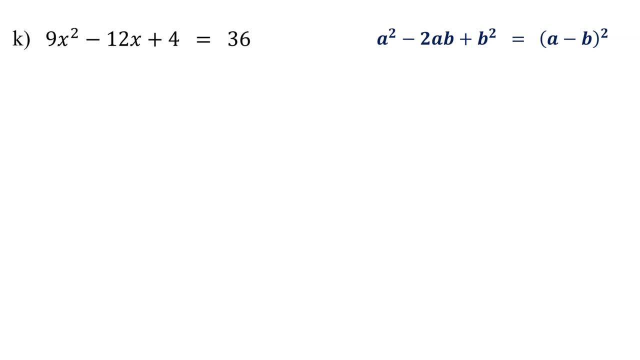 a squared minus 2ab plus b squared, which is equal to a minus b squared. 9x squared can be written as 3x squared right And 4 can be written as 2 squared. Therefore, the middle term is 2. 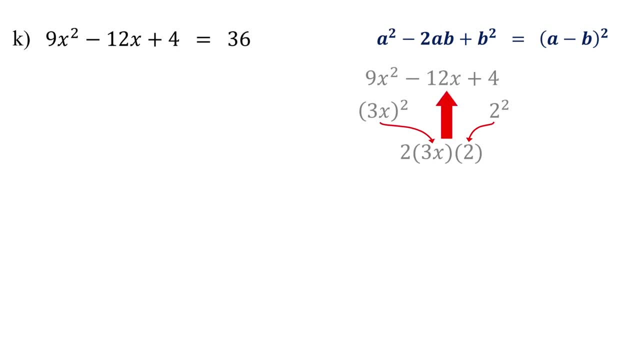 multiplied by 3x times 2, which equals 12x. This confirms that this trinomial is a perfect square, so we can factor it easily. Since a is 3x and b is 2, we can factor it as 3x. 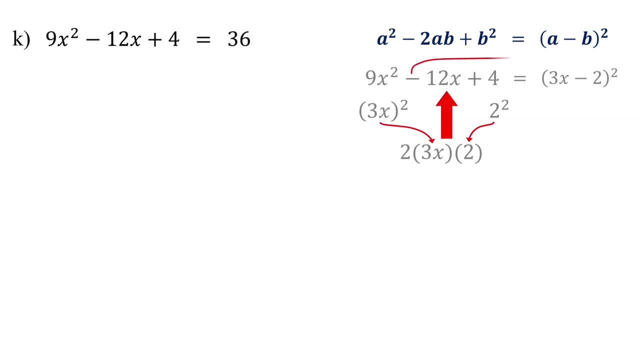 minus 2 squared. Remember, if the sign of the middle term is negative, the sign in the factor is also negative. Now apply the square root property. The square root of 36 is 6.. Next, set up the two equations and solve them. For the first equation, add 2 to both sides of the. 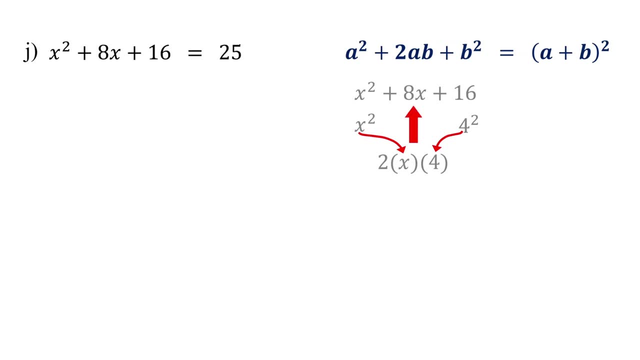 2 times x times 4 is 8x. Therefore, since all three conditions are met, this trinomial is a perfect square. Now, since a is x and b is 4, we can factor it as x plus 4 squared. 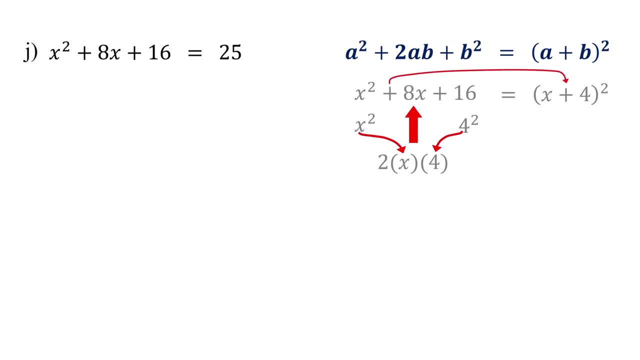 Notice that if the sign of the middle term is positive, the sign in the factor is also positive. Similarly, if it is negative, the sign in the factor is also negative. Now treat the whole binomial as a single variable and apply the square root property. 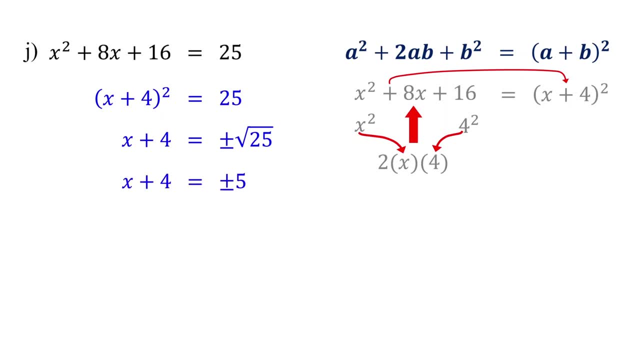 The square root of 25 is 5.. Next set up the two equations and solve them. From the first equation, we get x equal to 1.. From the second equation, we get x equal to negative 9.. Therefore, the two solutions are x equal to 1 or negative 9.. 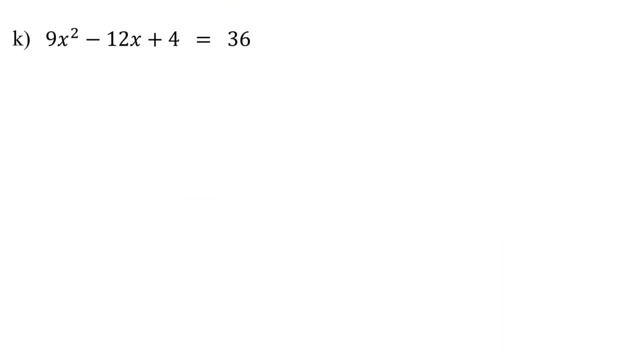 Let's do one more example like this. This is the final one, so please stay with me. Just as we did in the previous example, our first step is to factor the perfect square trinomial. This trinomial is in the form: 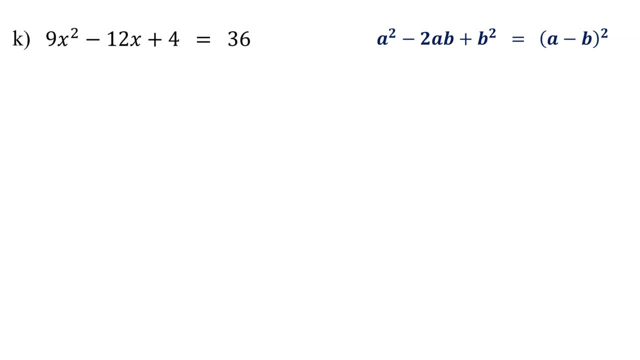 a squared minus 2ab plus b squared, which is equal to a minus b squared. 9x squared can be written as 3x squared right And 4 can be written as 2 squared. Therefore, the middle term is: 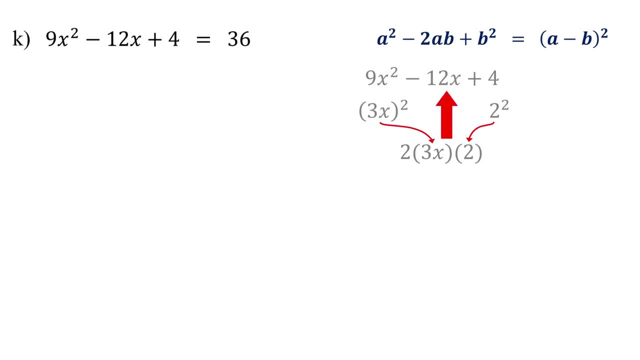 2 multiplied by 3x times 2, which equals 12x. This confirms that this trinomial is a perfect square, so we can factor it easily. Since a is 3x and b is 2, we can factor it as 3x minus 2 squared. 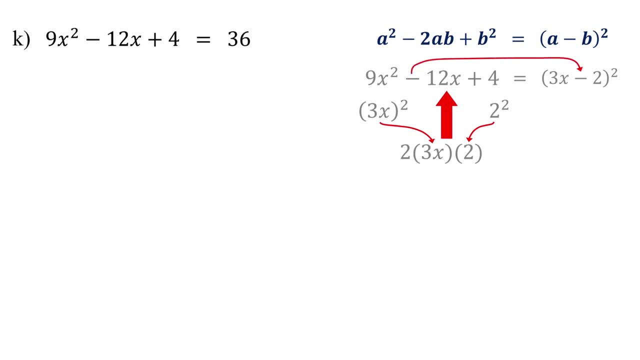 Remember, if the sign of the middle term is negative, the sign in the factor is also negative. Now apply the square root property. The square root of 36 is 6.. Next set up the two equations and solve them. For the first equation, 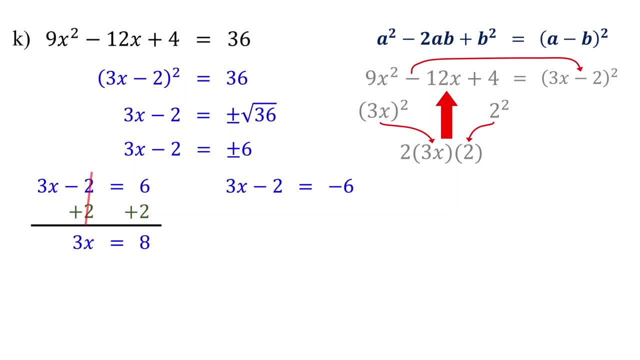 add 2 to both sides of the equation to isolate 3x. Then divide both sides by 3, and you get x equals 8 over 3.. For the second equation: again add 2 to both sides of the equation to isolate 3x. 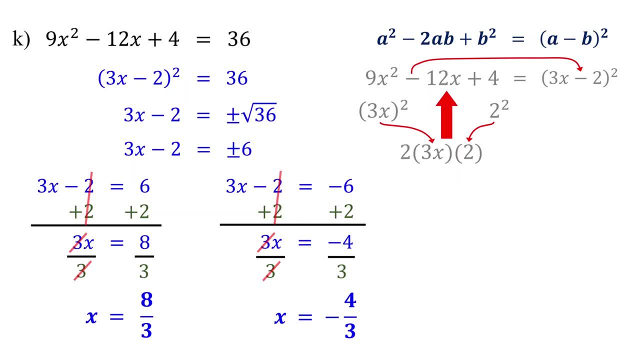 Then divide both sides by 3, and you get x equals negative 4 over 3.. Therefore, the solutions are: x equals 8 thirds or negative 4 thirds. Thanks for watching. If you found this video helpful, please give it a thumbs up and subscribe. 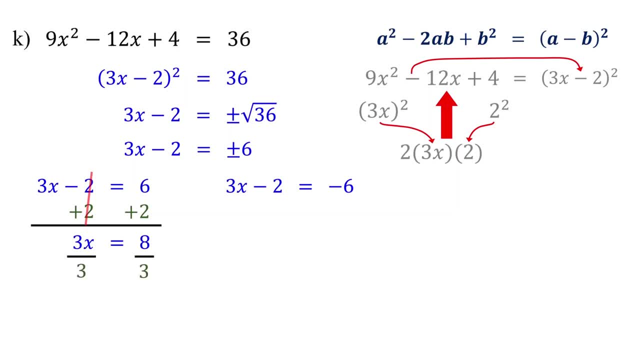 equation to isolate 3x, Then divide both sides by 3, and you get x equals 8 over 3.. For the second equation, again add 2 to both sides of the equation to isolate 3x, Then divide both sides by.